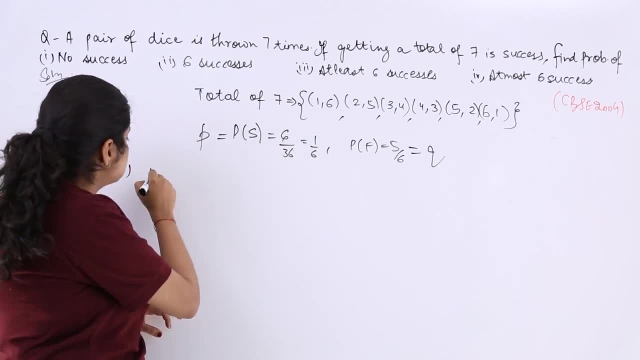 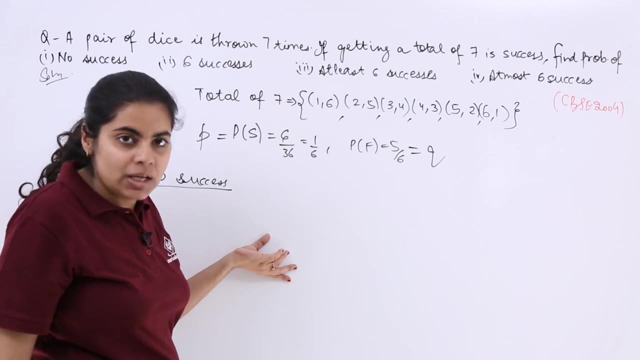 probability you have to take out of success is 6 over 36, which is 1 by 6.. So the probability of a failure is a success because you took out from zero times go over a ten. The first part says that the probability of na Roosevelt'sis less than 4 out of 17 is. 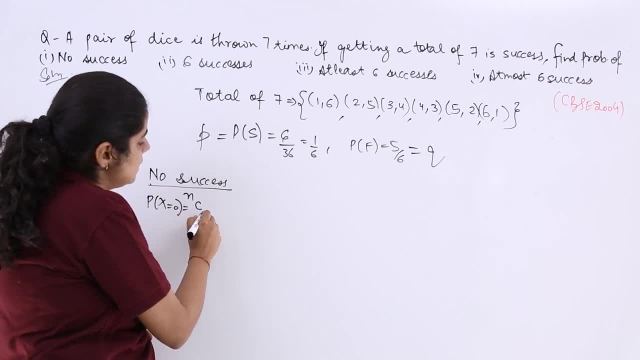 equal to 0. So, so, so, so- so, so-so, it is 0 if it is 0 or zero, It is 0 if it is 0. So one size fits the size. Anyways, you can take out for no success. So the first part, no success. 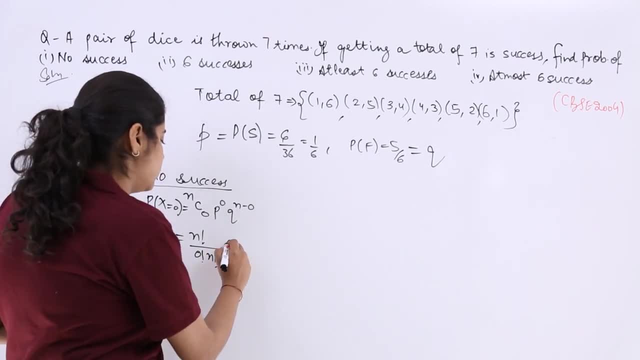 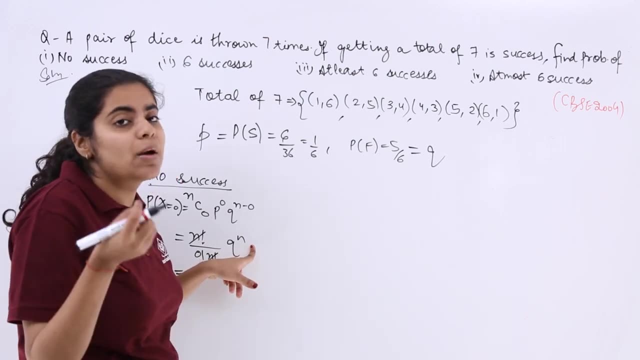 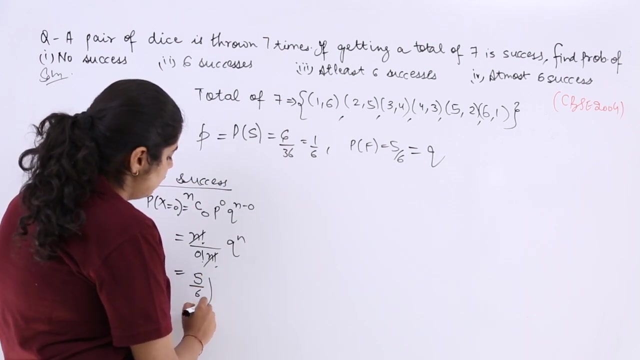 Now you know the simple formula and you can directly use that formula. Now: nCR, no success to the power n. So cancelling whatever cancels. Now q raised to the power n. What is q? q is basically the probability of failure. So it is 5 upon 6.. So this is 5 over 6 whole. 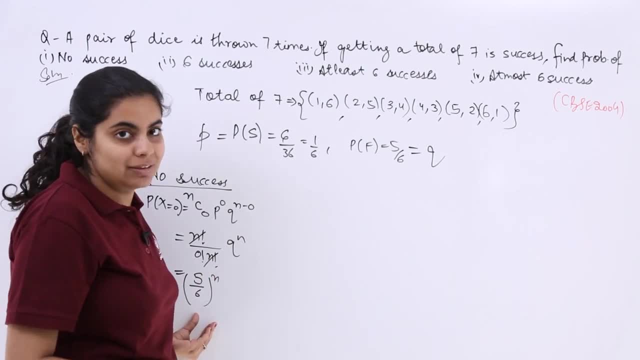 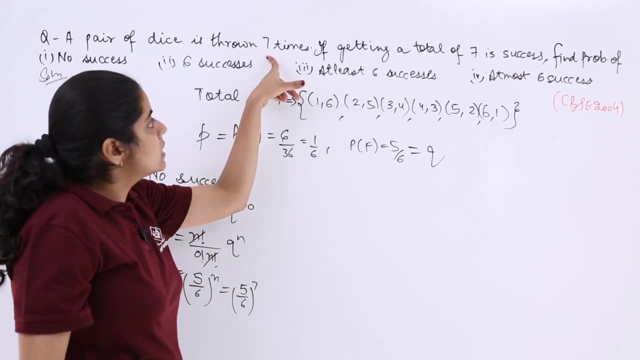 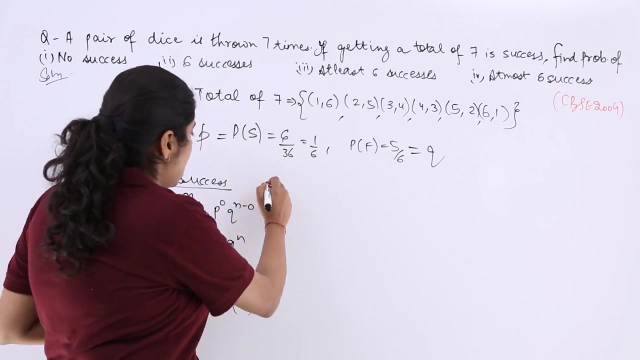 raised to the power n. So this is the first part. And here what is n? n is basically 7, because you have to get c thrown 7 times, So tossing is done 7 times. So n is number of trials which are 7.. After the first part, let's see the second part. So this is the 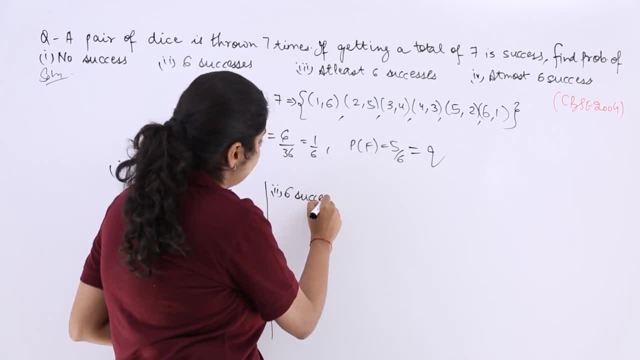 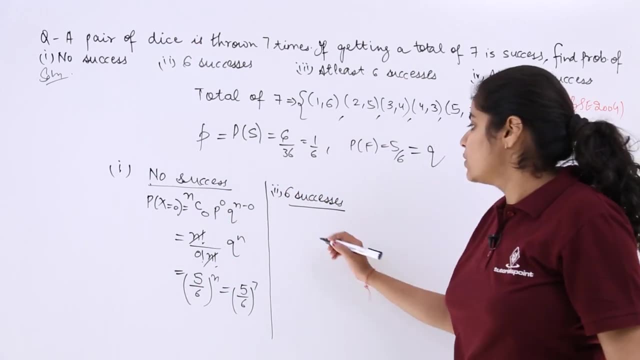 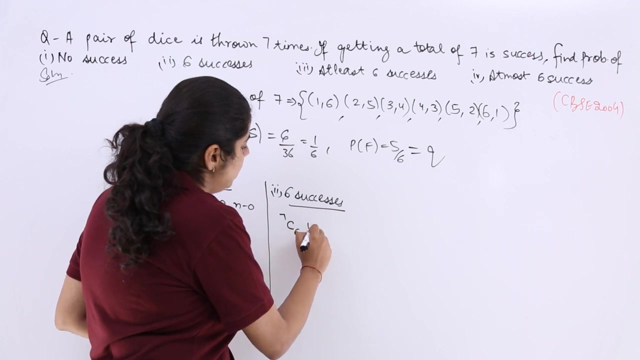 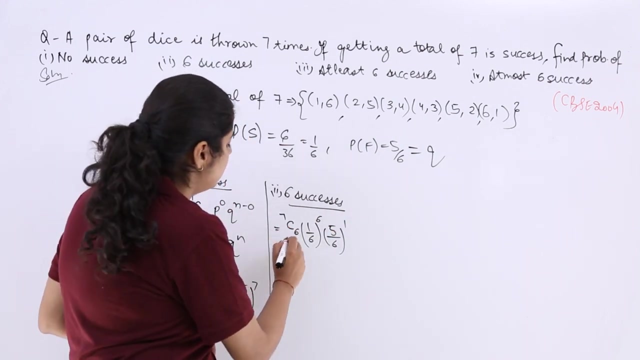 first part. The second part is 6 successes. So for 6 successes- I know the value of r is given to me as directly 6.. So it is ncr means 7 should be your n again. So ncr is p raised to the power r, q raised to the power n-r. Now 7c6 is basically 7c1.. Multiply: 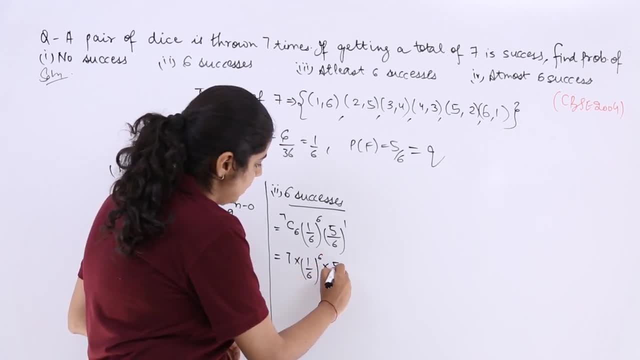 by 1 upon 6, whole, raised to the power 6.. Multiply by 5 upon 6.. So either you can leave your answer here or you can do 7, 5size, 35.. Multiply by 1 by 6, whole, raised to the power 7.. So. 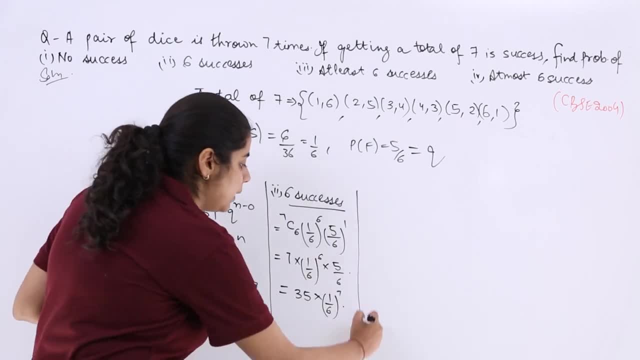 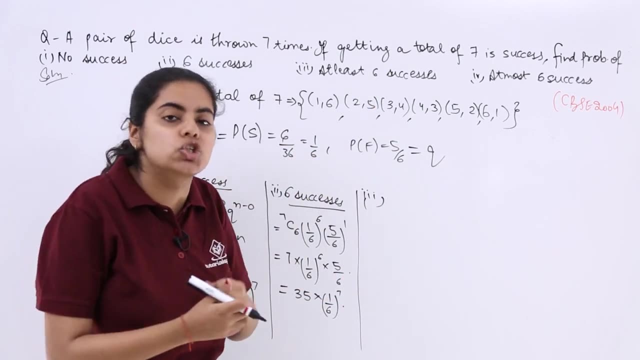 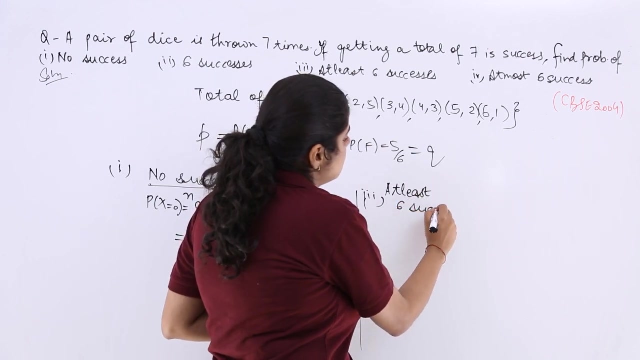 this is the answer to the second part. What about the third part? The third part is regarding at least 6 successes. So minimum 6 successes should come. So when I say at least 6 successes means minimum 6 successes, Minimum 6 successes means either: 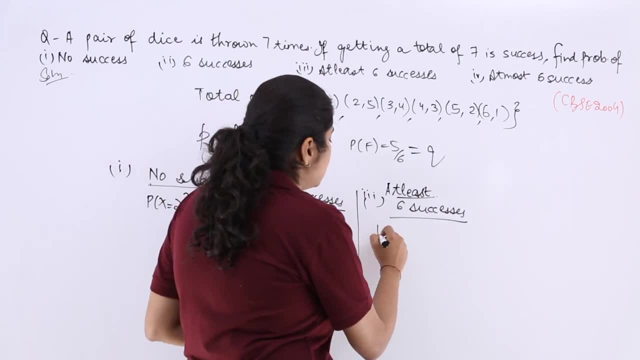 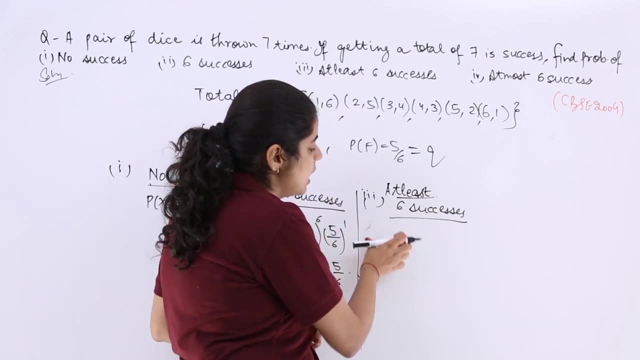 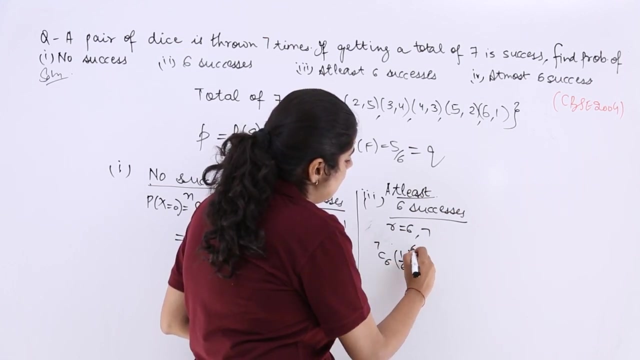 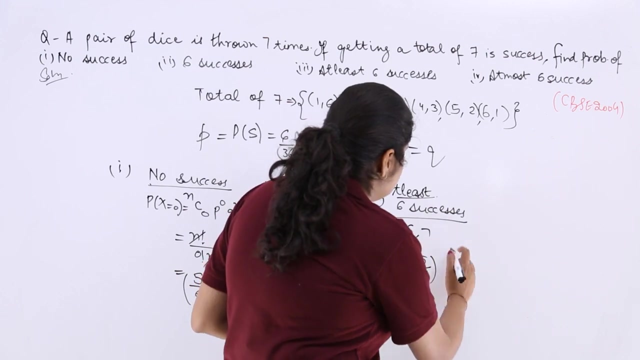 6 is the value of r or 7.. So it will be ncr. I erase it here because r can be both 6, 7.. So ncr. p raised to the power r, q raised to the power n-r. So this is there Also. I know that at least means one more thing has. 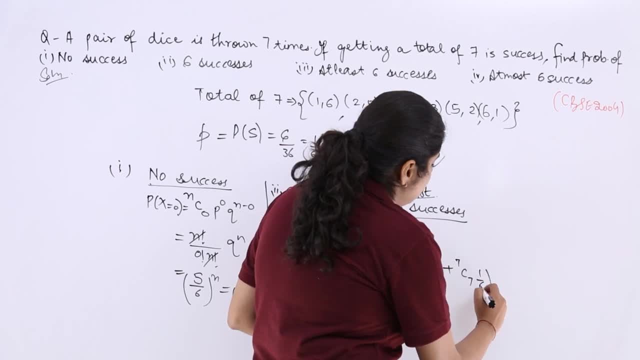 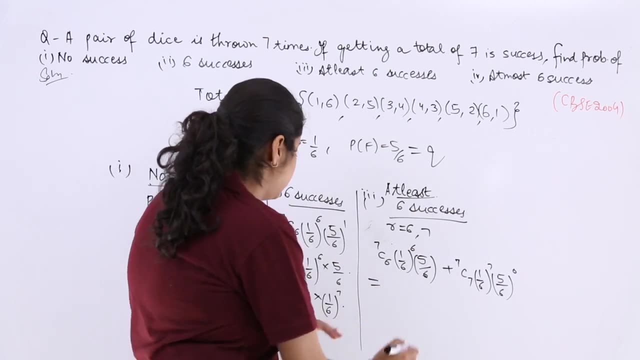 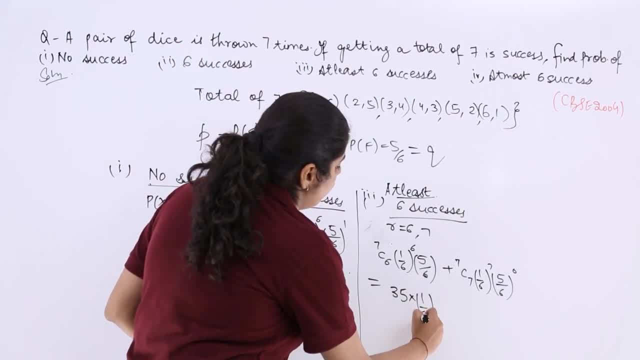 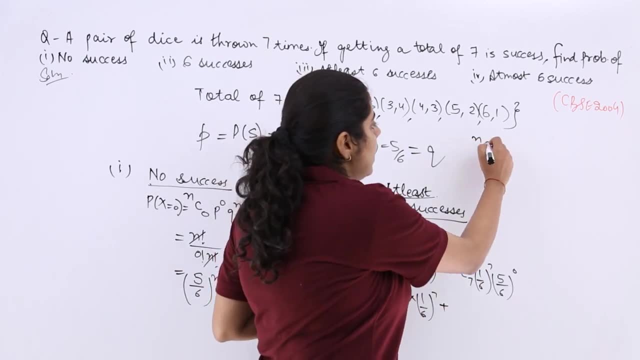 part, which is 35, multiplied by 1, by 6 whole raise to the power 7.. Here what I can do is I know what is 7c7, what is ncnc. ncn is n factorial upon 0 factorial into n factorial. 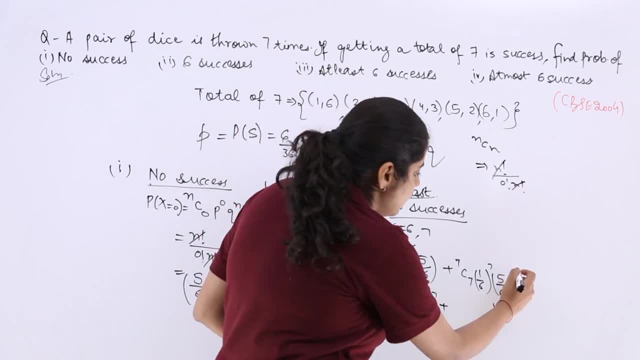 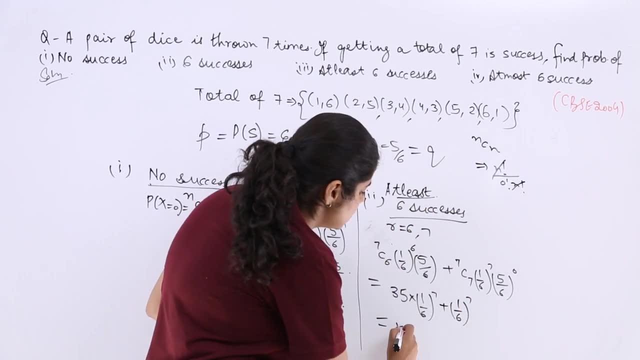 which is 1.. So this is ignored completely. and this because raise to the power 0 is already 1.. So this is 1 by 6 whole raise to the power 7.. So what you can do is 1 by 6 whole raise. 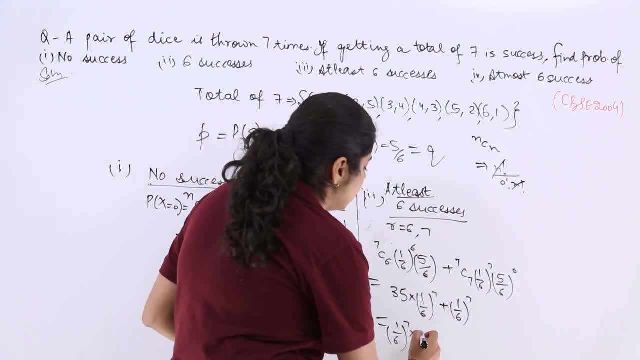 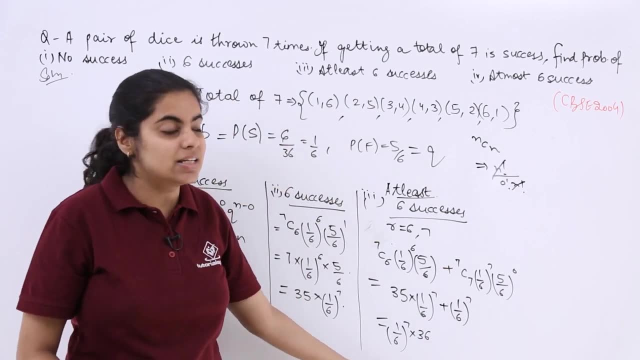 to the power, 7 can be taken as common, So that becomes multiply by, because since this can be taken as common, so 35 plus 1 is 36.. So these are the different answers to all the three parts. Now again, some people will find: 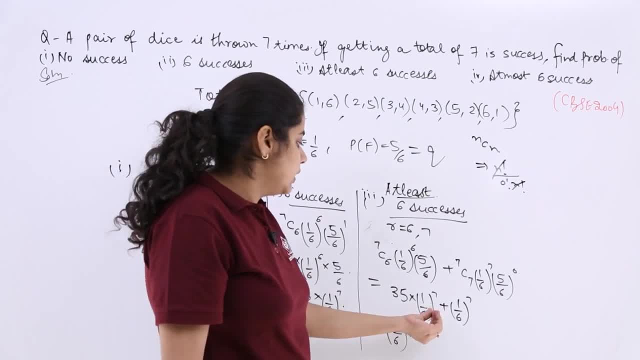 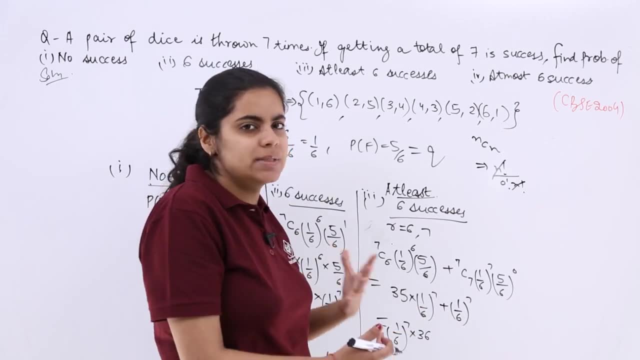 that I don't want to leave the answer like this. For me, probably this 1 by 6 whole raised to the power 7 is not use of me. What I'll do is I'll just take something common and then divide into lowest terms. It's up to you how you simplify. The main answer is after this step. If you don't, 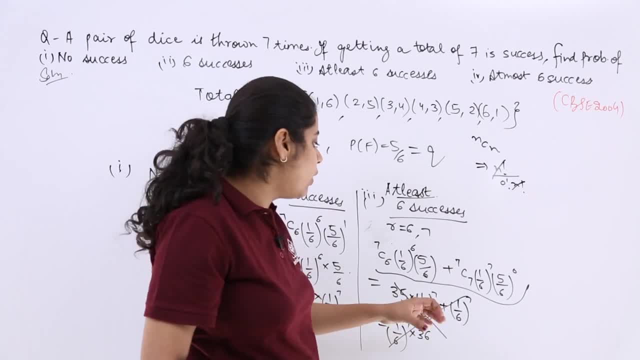 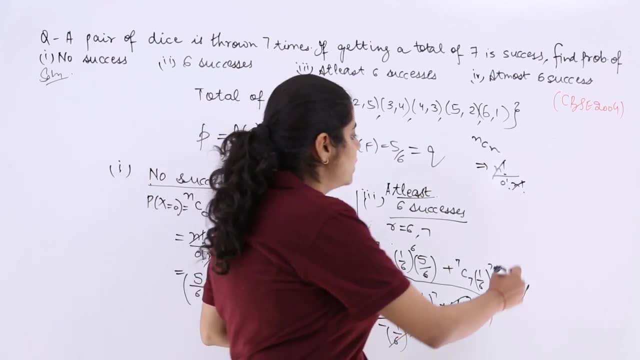 want to follow this. you can anyways change it and do the way you want. What you can do is you can take 1 upon 6 whole, raised to the power, 6 common, and then accordingly, the answer will change. for the simplest terms, What is the fourth part? regarding The fourth part is at most 6.